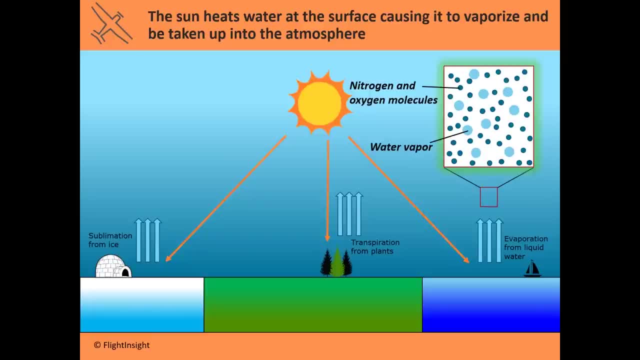 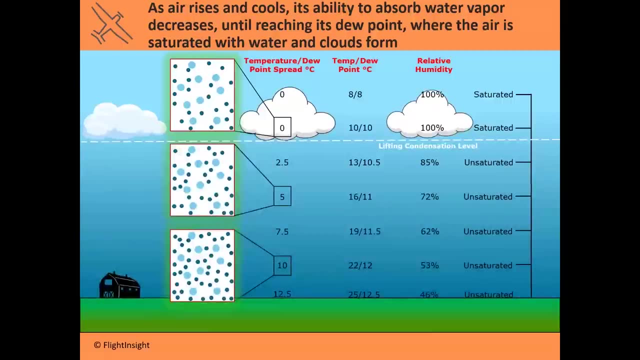 liquid water vaporizing as the sun warms it up. So all three of those processes are going to introduce water vapor into the atmosphere. Okay, now, we don't usually notice water in the atmosphere. You typically can't just wave your hand around and then come up with small water. 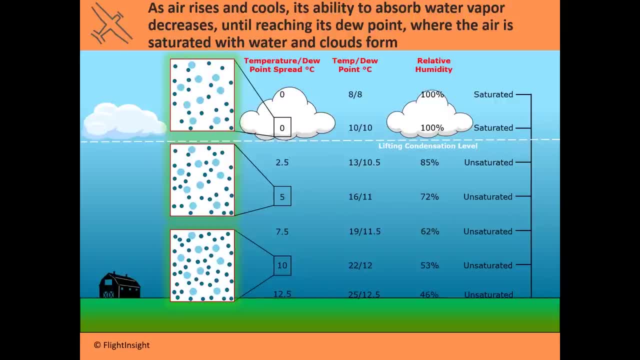 droplets on your hand from the atmosphere. So where is that water? It's being absorbed into the atmosphere. It's almost as if that water is dissolving into atmosphere, the same way your sugar dissolves into your coffee in the morning if you take it with. 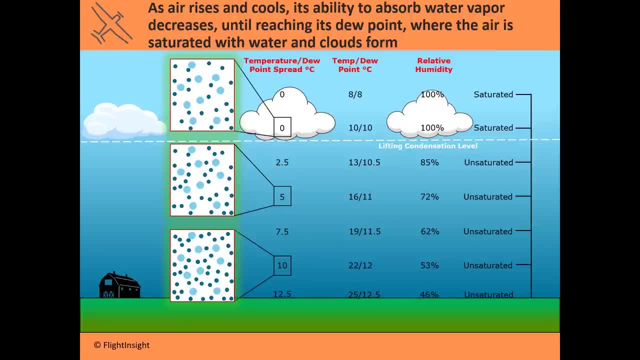 sugar. A little bit of what you've put into the atmosphere is absorbing into it. but the air can only absorb so much of that moisture. At a certain point it's become saturated. It can't take any more of the moisture and that moisture has to go somewhere. Where it goes, is it condenses, onto what? 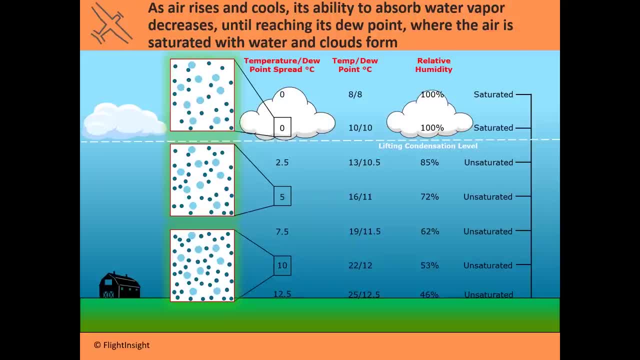 are called condensates. So what we're going to do is we're going to take the condensation nuclei in the atmosphere, particulate matter, dust, carcinogens from the stuff that we're burning on the surface, anything that's up there. 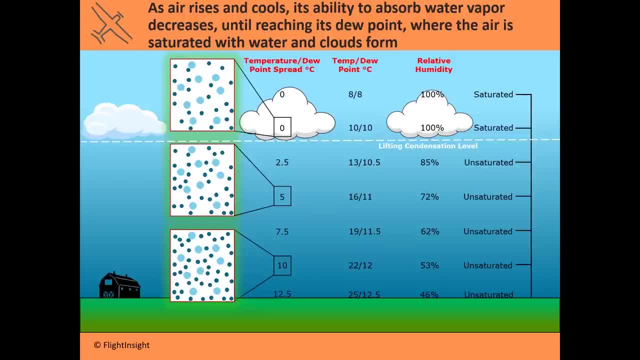 in the sky can have water condense around it. This is where clouds come from. Clouds will happen. Clouds will form if the air isn't able to absorb any more moisture and it's got to sort of park it somewhere else. Now, the ability of air to absorb moisture, the ability of air to absorb water is 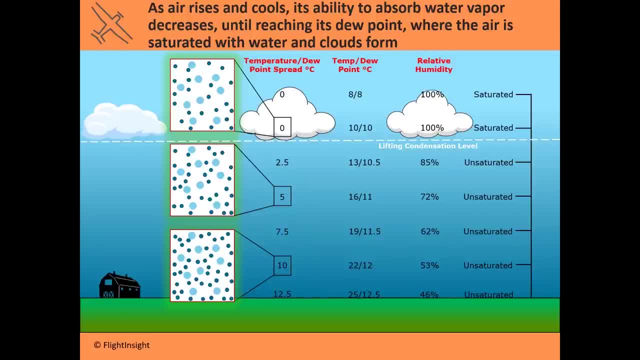 related to its temperature. You can think of the coffee metaphor again here. right? You know I love Dunkin' Donuts. I don't know about where you get your morning coffee from, but I love going to Dunkin', And what I used to do, especially in the summer months, was I'd get an iced coffee instead of a hot. 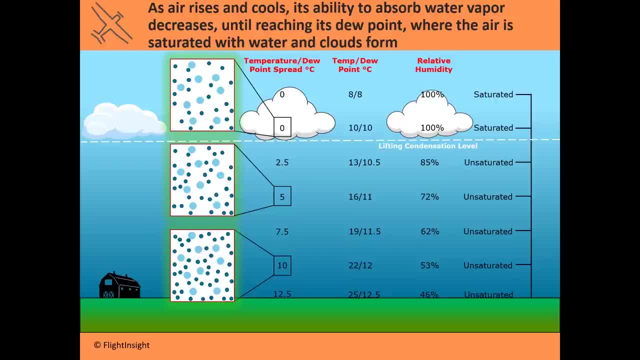 coffee, And if you know Dunkin' Donuts, you know that they put a lot of sugar in your coffee. For me it's too much sugar, but when I was younger I didn't mind having so much of that sugar in there. but they 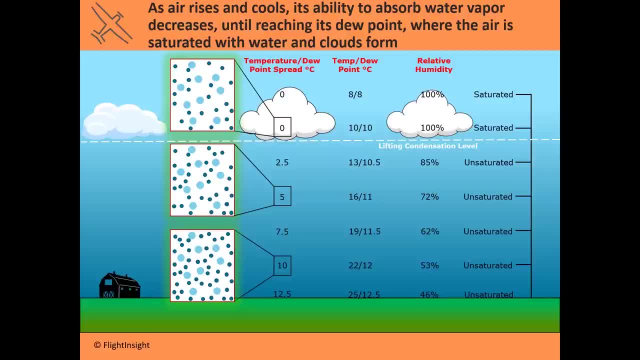 really load it up And what you notice is that in the iced coffee. you take a sip of that iced coffee and you're going to notice that there's little bits of sugar hitting your tongue. You can actually feel the granular sugar, Whereas when you get a hot coffee and they put 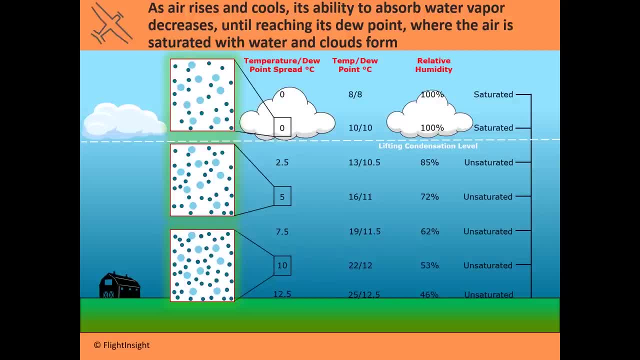 that same massive amount of sugar in there. you don't notice it. You notice how sweet it is, You notice the taste, but you don't notice the actual feel of the grains of sugar in there. So it's the same amount of sugar. In the case of the atmosphere, it's the same amount of water vapor that's going in there. but because 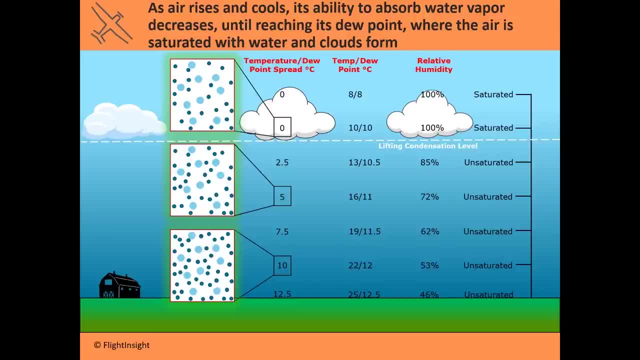 coffee in my case. air, in the atmosphere's case, has gotten colder. the ability of it to absorb whatever you've put into it is reduced. So the colder air becomes saturated a lot more easily. You can't hold as much moisture at colder temperatures. The iced coffee can't hold sugar. The colder atmosphere can't hold as much moisture. So what? 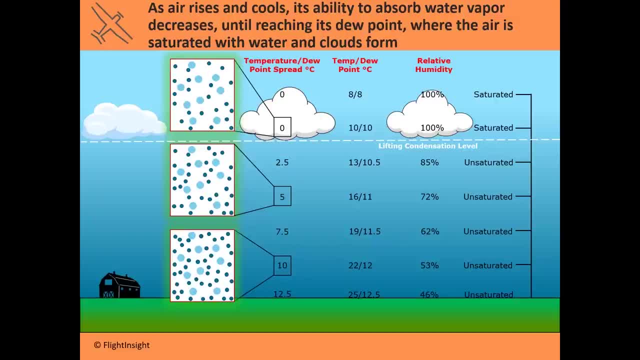 goes on, is that as temperatures drop, they get close to what's called their dew point, the temperature that, if they fall to, the air will be saturated. It will no longer be able to hold any more moisture, and it's at that temperature that clouds will form. So what you see in 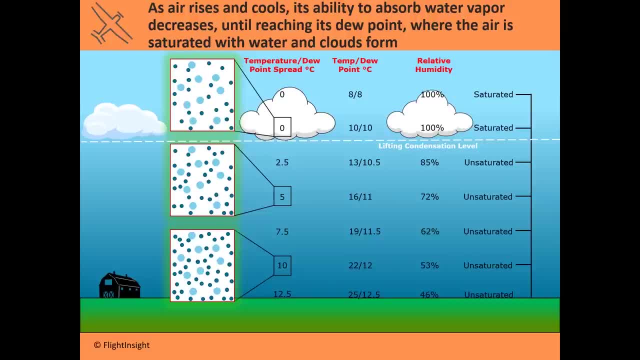 this image here is: you see, starting at the surface. you have basically a column of air that starts at the surface and we have three columns to describe what's going on in the air. The first one is the temperature dew point spread. This is the difference between the temperature of the air and its dew point. And then you see in that second column what those 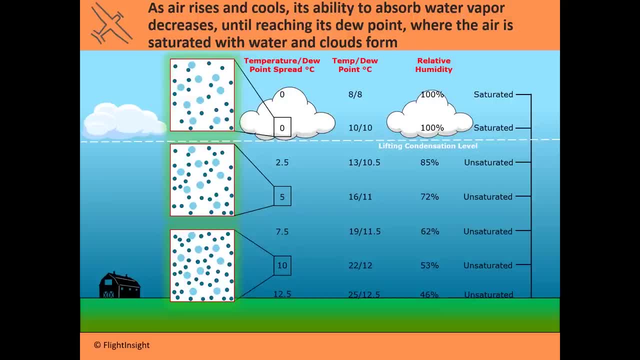 temperature and dew points are: It'll be 25 Celsius and 12.5 degrees for the dew point. So the spread is just: you take that temperature at 25 and you subtract the dew point at 12.5 to get a spread of 12.5.. This is the difference between the 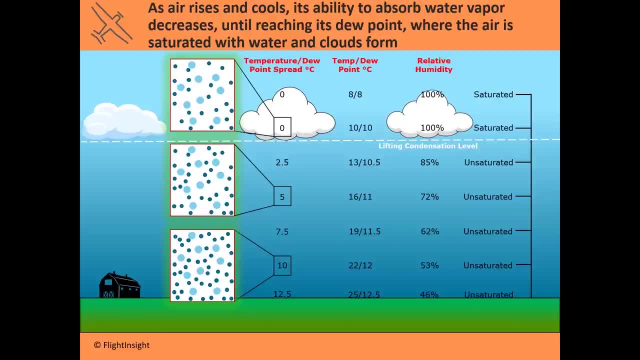 temperature and the dew point, And it is related to something called relative humidity, which is how far away that air is from being fully saturated for having the formation of clouds. Now remember, air cools as it rises and there's a rate that 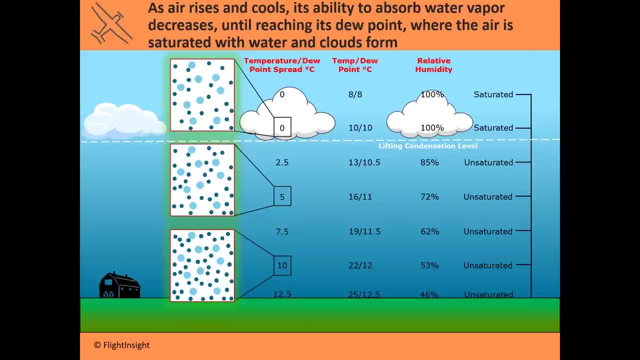 air cools at as it rises. The rate that it cools at depends on if it's dry or moist air. In other words, it depends on if it's saturated or unsaturated. So there's fancy terms for this: dry adiabatic rate and wet adiabatic rate. We're not going to get into that.